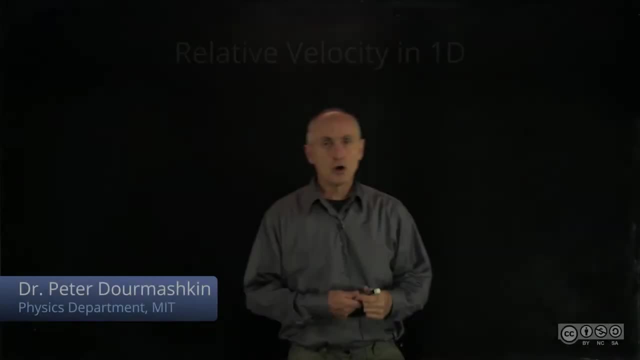 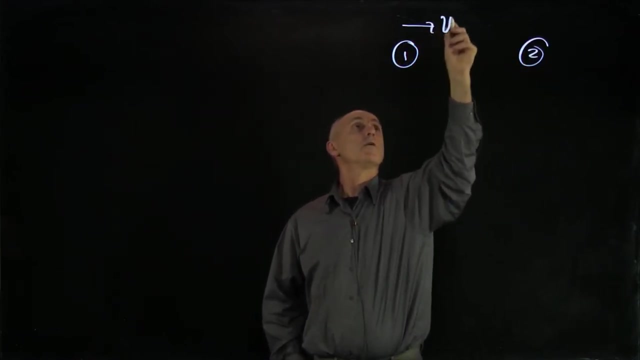 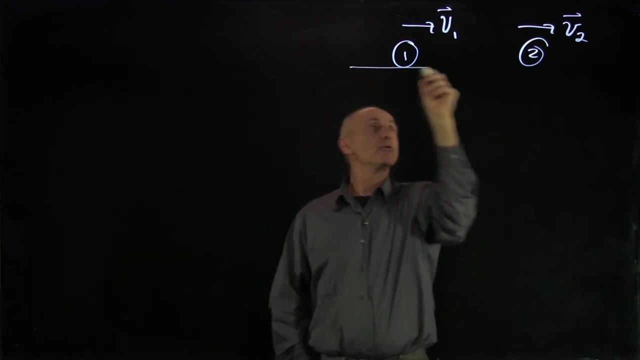 For one-dimensional collisions. let's talk about two objects, one and object two, moving with velocity v1 and another object, v2, moving with velocity v2.. Let's say they're moving on the ground. Now I'd like to introduce the concept of relative velocity, a concept 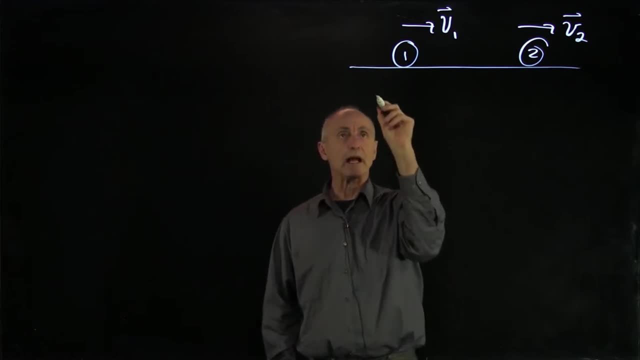 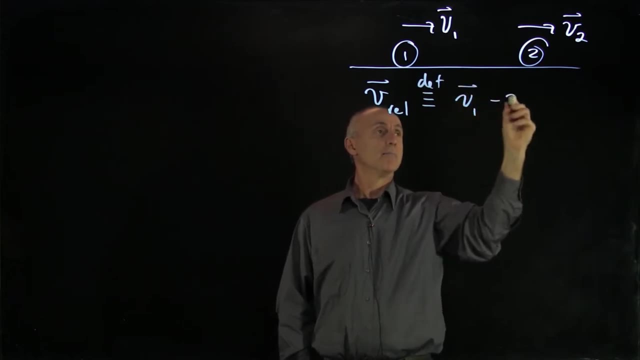 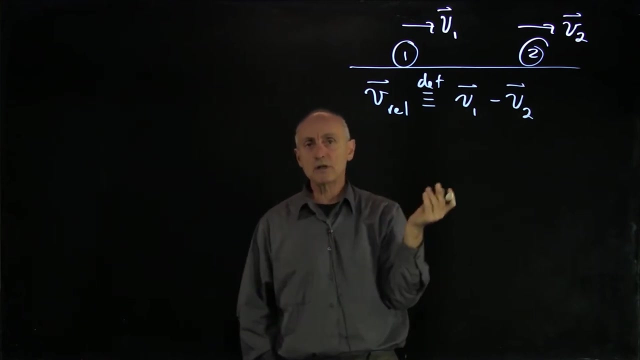 that we experience all the time in our lives. but let's see what it actually means. So v relative. I'm going to define this to be the velocity of one minus the velocity of two. Now, because of this minus sign, that seems a little bit abstract. but one typical example. 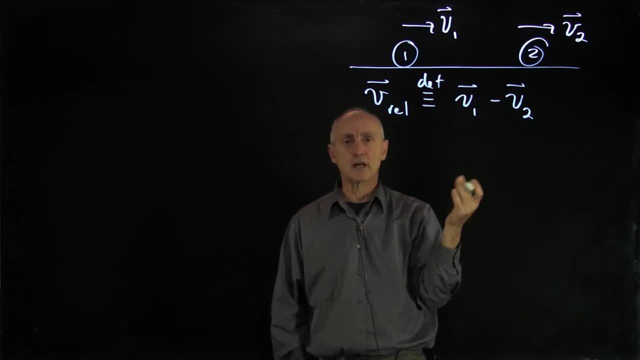 where we see this all the time is for people traveling on highways. You might have two cars, one car overtaking the other car, but if you're sitting in car one, it looks like car two is going quite slow. So let's just take a typical highway example. So you're 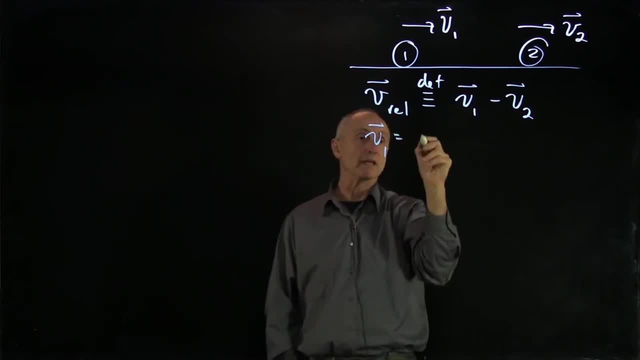 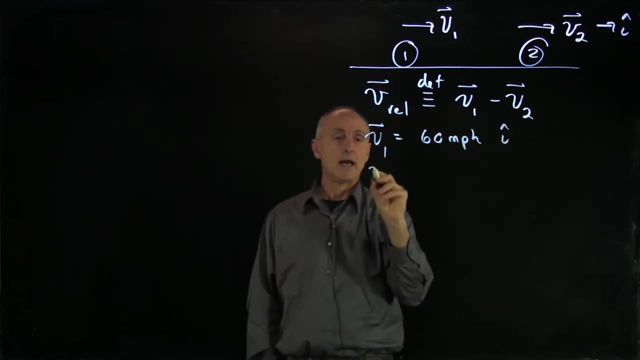 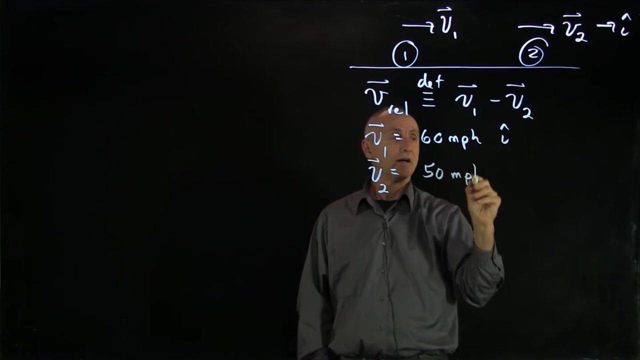 going to have v1, and we'll give this some speed, so we'll make it 60 miles per hour and we'll just call this one-dimensional problem. i hat and v2, notice we're not speeding on a highway. v2 is going at 50 miles per hour. i hat very slow And the relative 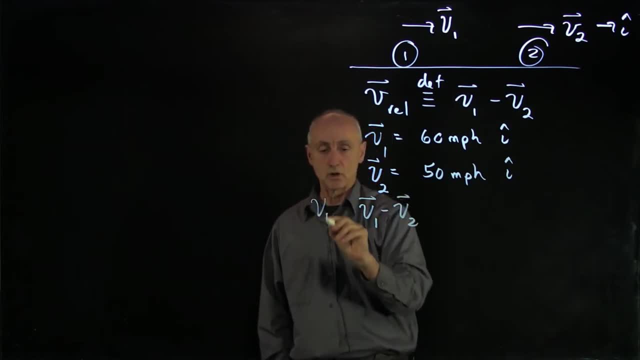 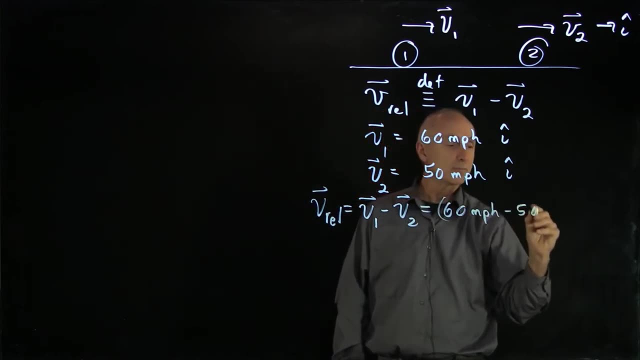 velocity: v1 minus v2, so that's what we're calling v relative. that's 60 miles per hour minus 50 miles per hour i hat, and that's just 10 miles per hour. and that's what people 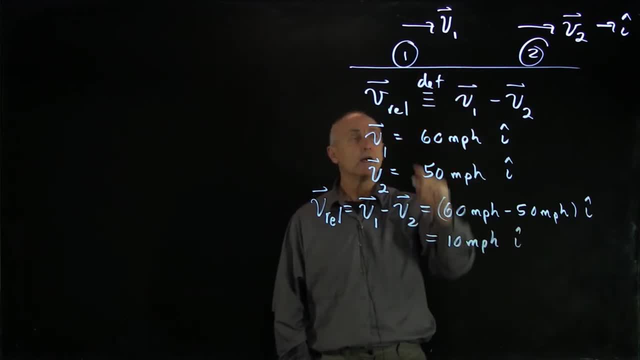 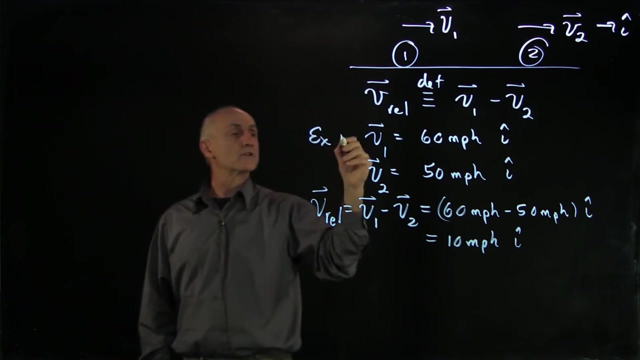 experience when one car is approaching another car. If you're in car two, car one seems like it's coming at you at 10 miles per hour. This is what we mean by relative velocity. There's another important example. so that's example one. The other important example to look at: 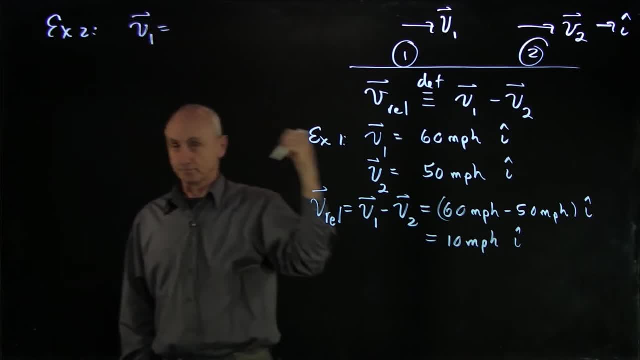 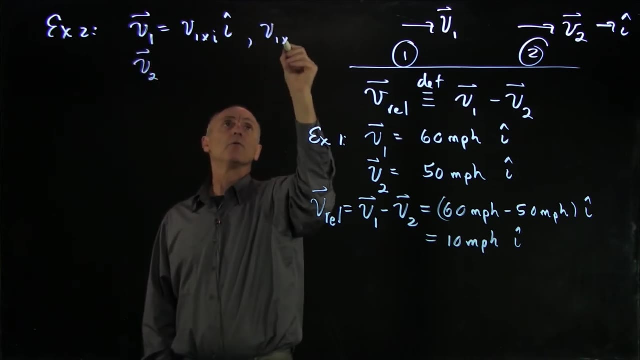 example two is when two objects are moving in opposite directions. So let's just write here a. let's write them in terms of components this time. So we have v1, x1, and we have v2, and let's make v1, x positive.